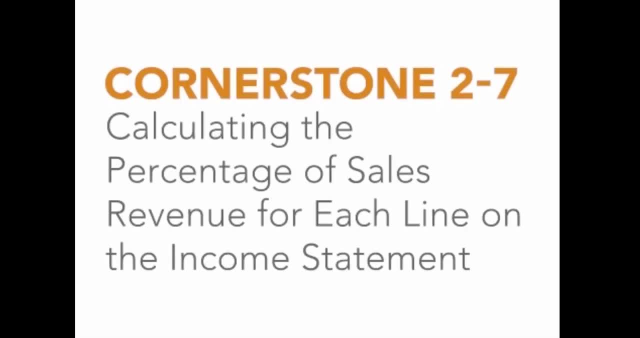 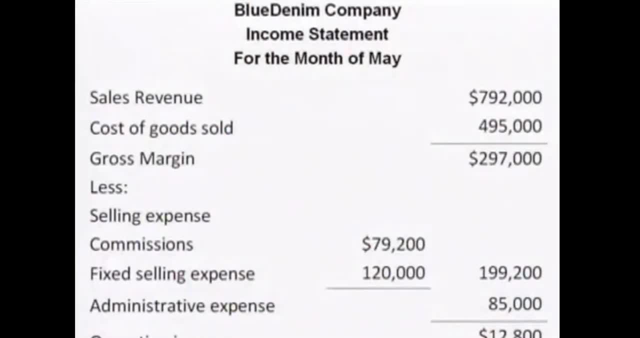 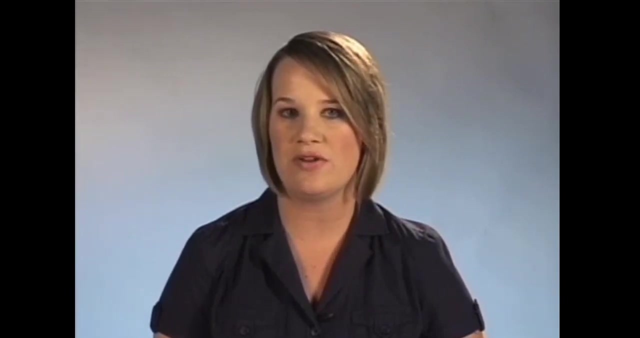 Recall that in the previous cornerstone we prepared the Blue Denim Company's income statement for the month of May, which is provided here In this cornerstone. we are asked to use the income statement to calculate the percentage of sales revenue represented by each line of the income statement. 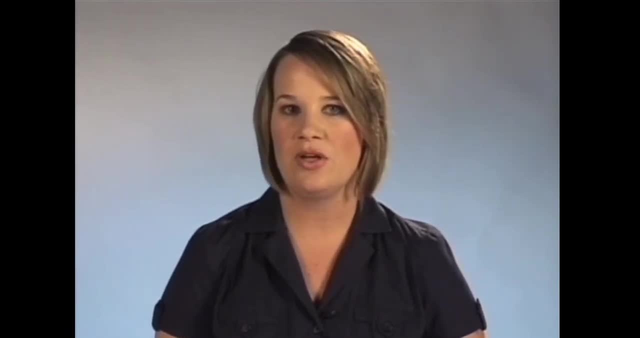 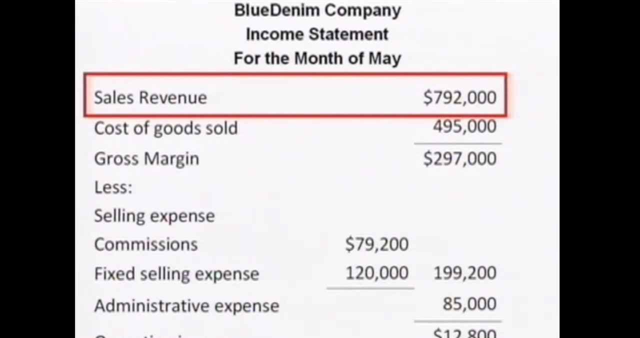 To calculate the percentage of sales revenue, we will always take the line of the income statement that we are calculating the percentage for and divide by the sales revenue. For example, to calculate the sales revenue percent, we would divide the line item of sales revenue by sales revenue or 100%. 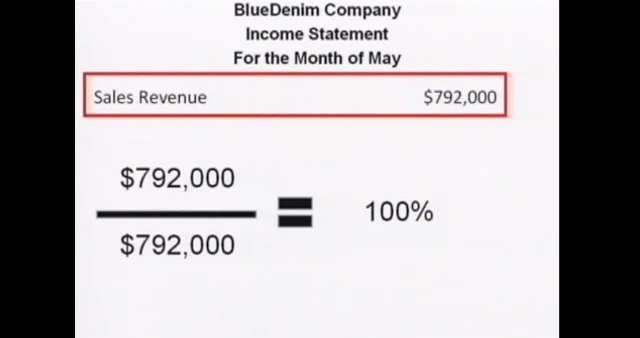 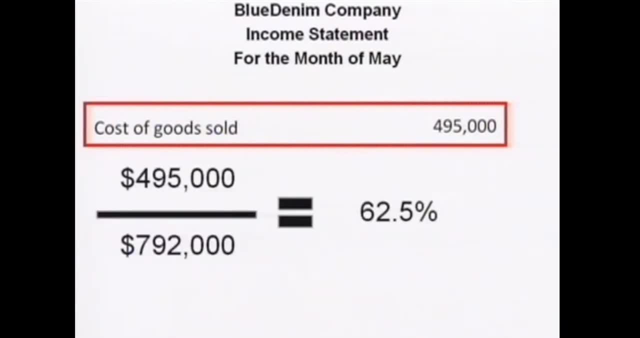 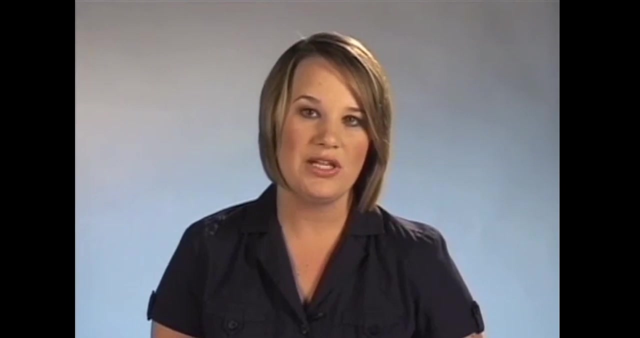 Notice that sales revenue is always 100% of itself. The cost of goods sold percentage would be calculated as the line item of $495,000 divided by sales revenue, $792,000, equaling 62.5%. All remaining percentages would be calculated in a similar manner. 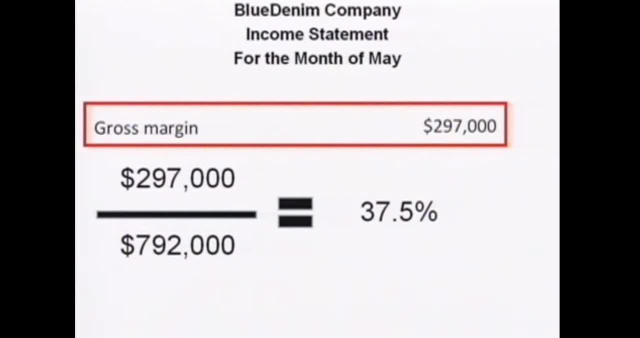 Gross margin percent equals $297,000 divided by $792,000.. Gross margin percent equals $297,000 divided by $792,000. Or 37.5%. Selling expense percent equals $199,200 divided by $792,000, or 25.2%. 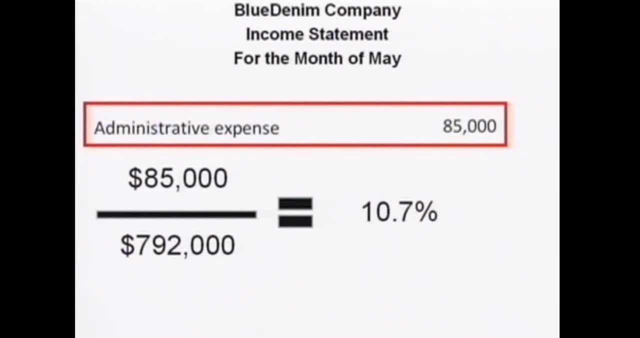 Administrative expense percent equals $85,000 divided by $792,000, or 10.7%. And finally, operating income percent equals $12,000.. Operating income percent equals $12,000.. Operating income percent equals $12,000. 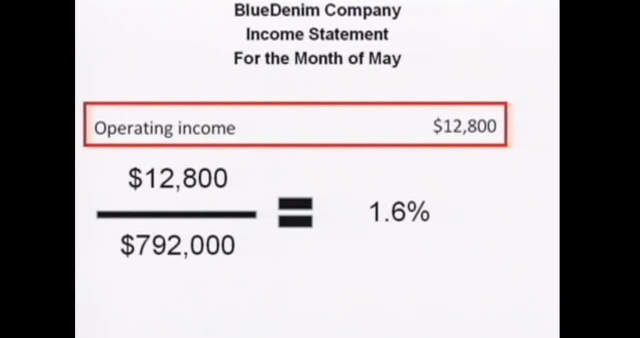 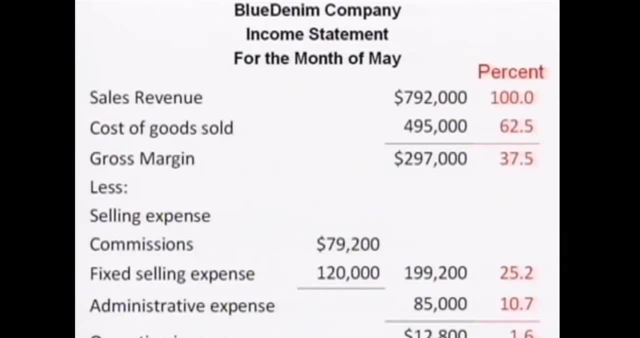 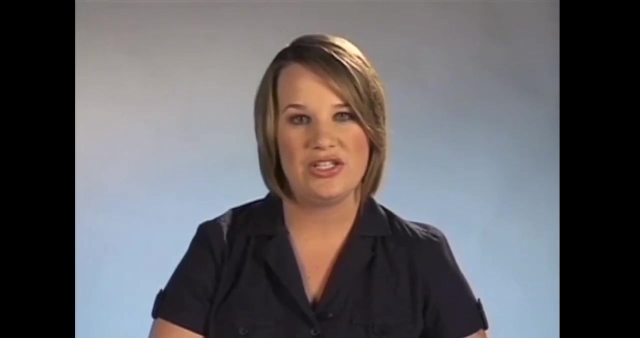 divided by $792,000, or 1.6%. In closing, let's review the income statement for Blue Denim Company and the percentage of sales revenue represented by each line of the income statement. These are marked in red. As you review these calculations, take a moment to think about.